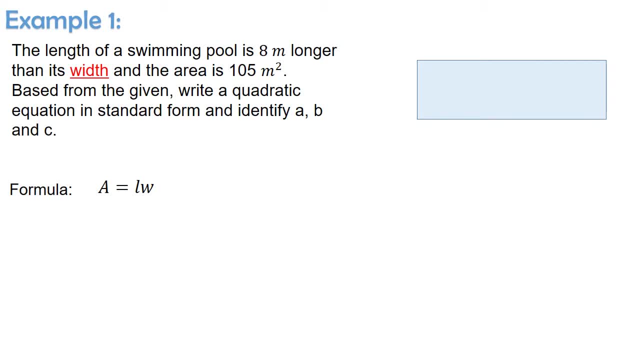 In this case, we will represent the measure of the width as X. So if we have the width as X meters and the length is described as 8 meters longer than its width, then we have X plus 8 meters as the length. Hence we now have the following given: 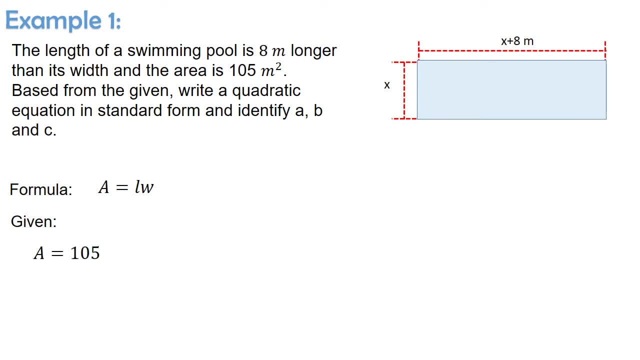 Area represented by capital A is equal to 105.. Width, represented by lowercase w, which is equal to 0.. Width represented by capital X and length, represented by lowercase l, which is equal to X plus 8.. 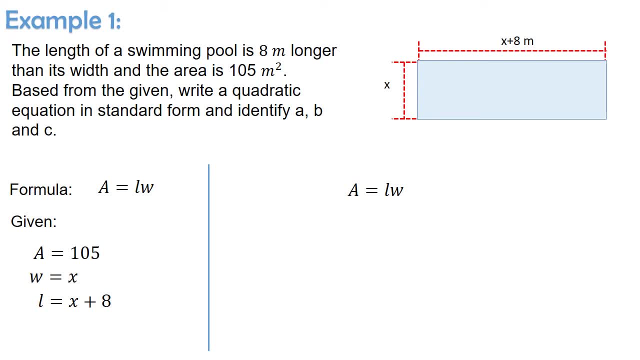 From here we just need to substitute this, given to our area formula, That is, 105 is equal to X times the sum of X and 8. Then we will just copy 105 on the left side of the equation and on the right side. 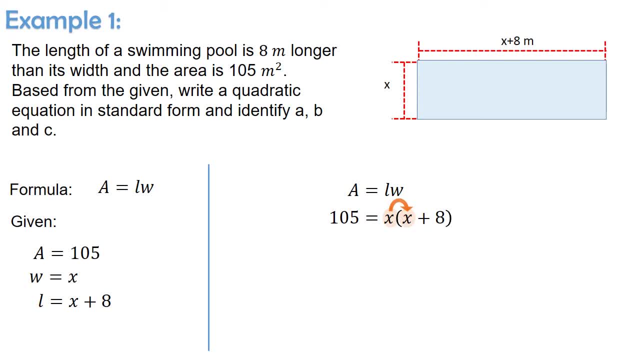 By applying the distributive property we have: X times X equals X squared and X times 8 equals 8X. From here we can already identify the quadratic, the linear and the constant terms. But what we need to do now is to apply APE to change our equation to standard form. 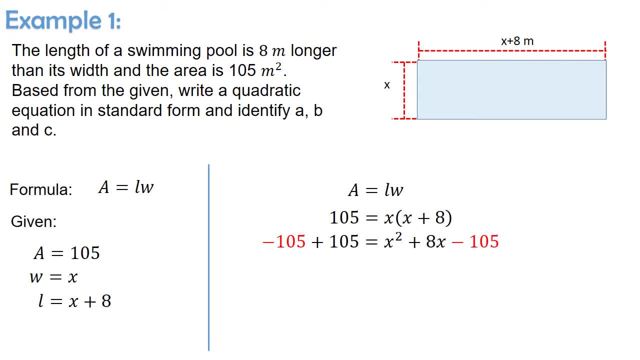 That is Subtracting 105, Subtracting 105 to both sides of the equation will give us 0 on the left side, and since we have nothing there to combine with negative 105 on the right side, then we have X squared plus 8X minus 105.. 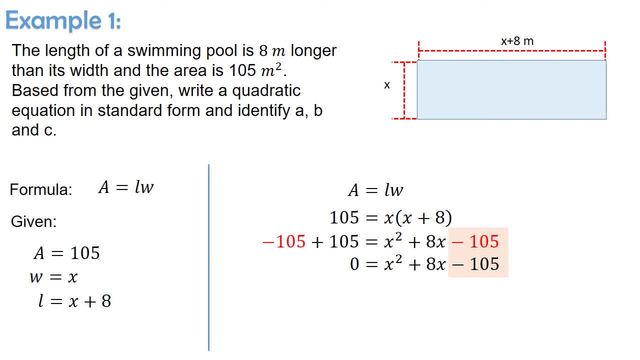 By the reflexive property of equality, we can say that 0 is equal to X squared plus 8X minus 105, is also equal to X squared plus 8X minus 105 is equal to 0.. From here, we can now easily identify the values of A, B and C of the standard form of the quadratic equation. 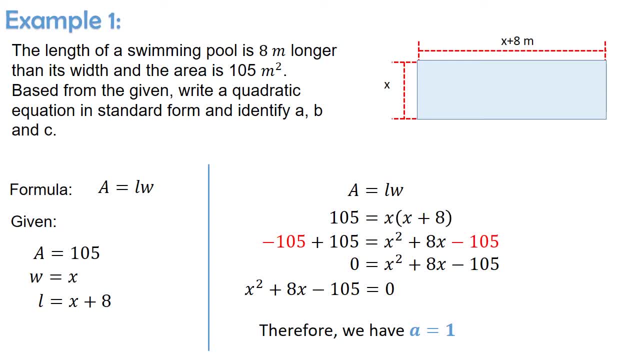 Therefore we have: A is equal to 1.. Take note if you can see any numbers beside a variable, it means its coefficient is 1.. B is equal to 8 and C is equal to negative 105.. Reminders: do not disregard the sign before the term. 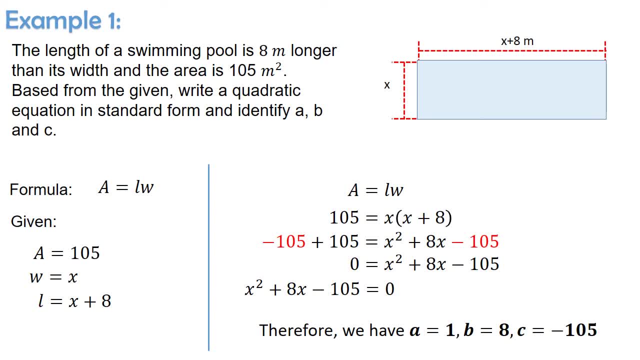 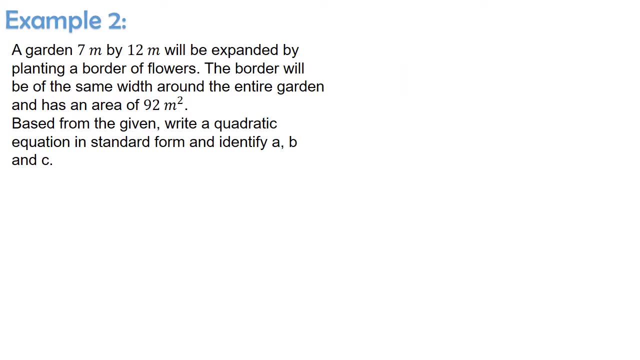 And there we have our first example. Let us have another example. Example 2 deals with a garden that we need to extend or expand. So let us create a model to help us solve the problem. Based on the given problem: we have a 7 by 12 meter garden and that we like to expand it. 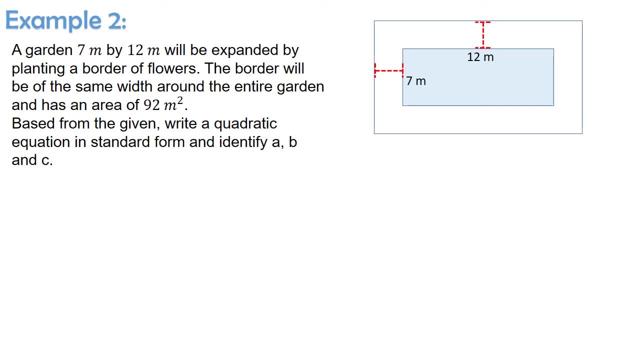 The border will be of the same width around the entire garden, But we don't know the length of the extension yet, so we represent the measure of the extension as X. Again, the problem involved an area, And we all know that the formula to solve area is. 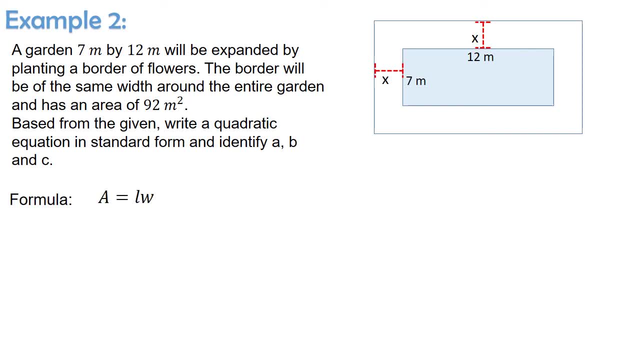 A is equal to length of the extension. B is equal to length times the width. Based from the problem, we have: L, which stands for the length, is equal to 12.. W, which stands for the width, is equal to 7.. Take note that we will expand the garden with the same unknown measure of width around it. 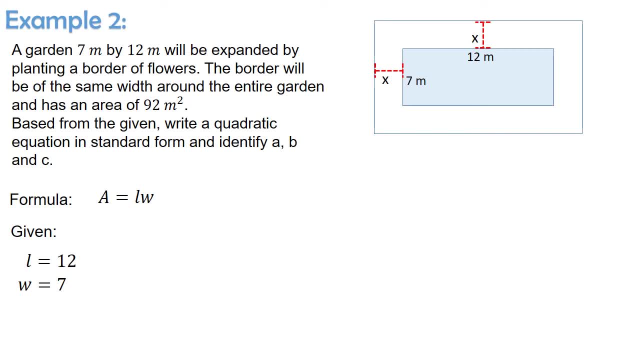 Adding this unknown measure to the length and width of the garden we have, L is equal to 12 plus 12.. W is equal to 7 plus X And W, which is equal to 7 plus X, And that from adding these unknown measures. 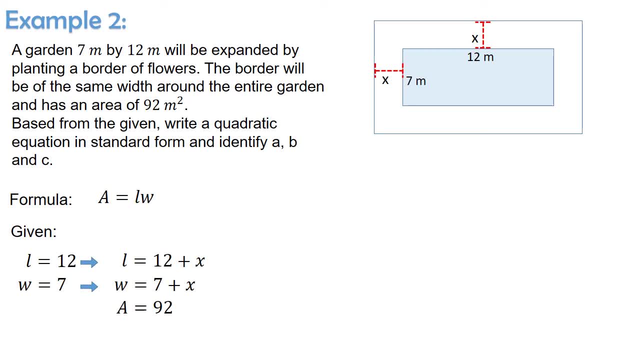 the garden will have an area of 92 square meters, And these measures are the new dimensions that we will use to solve the problem From here. we just need to substitute these, given to our formula, That is, 92 is equal to the sum of the length of the extension. 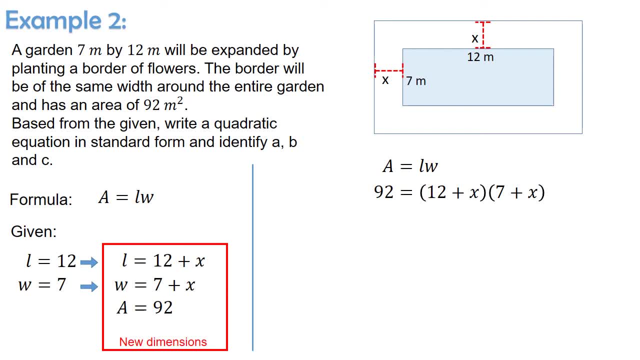 That is, 92 is equal to the sum of the extension. That is, 92 is equal to the sum of X and 12 multiplied to the sum of 7 and X. On the left side of the equation we will just copy 92.. 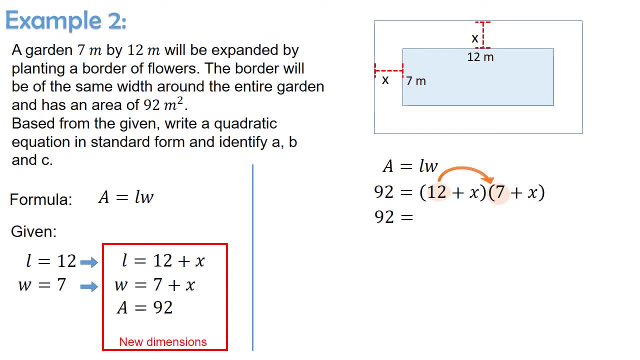 And then on the right side, by applying the distributive property or the FOIL method, we have: 12 times 7 equals 84.. 12 times X equals positive 12X. Positive X times 7 equals positive 7X. 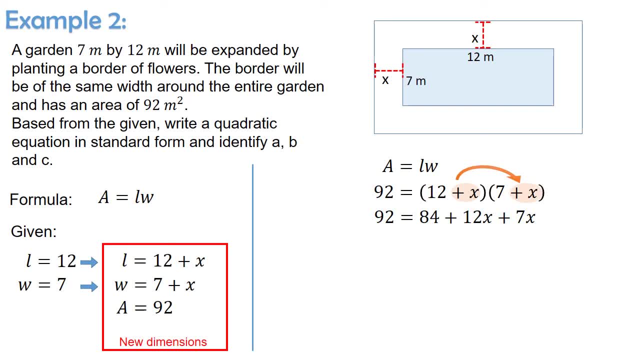 And positive X times positive X equals positive X. squared Adding like terms, we have 12X plus 7X, So we have positive 19X. From here we need to apply APE To combine like terms 92 and 84.. 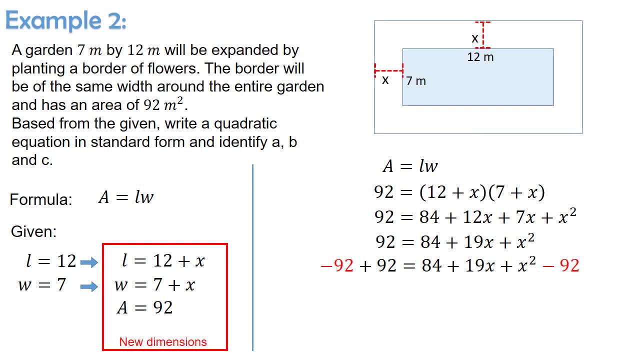 That is, subtracting 92 to both sides of the equation will give us 0 on the left side, And 84 minus 92 will give us negative 8 on the right side. So we have: 0 is equal to negative 8 plus 19X plus X squared. 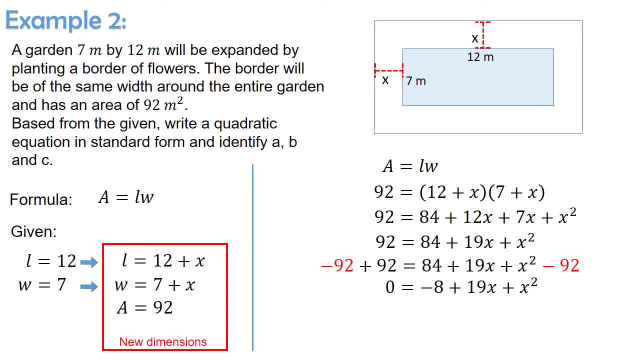 By the reflexive property of equality, we can say that 0 equals negative. 8 plus 19X plus X squared is also equal to X squared plus 19X minus 8 is equal to 0.. Note that we just rearrange the terms so that we follow the standard form. 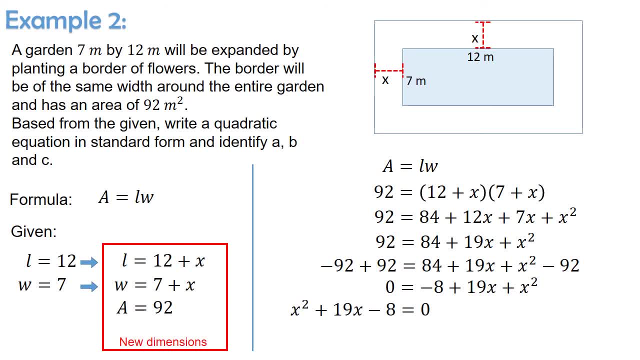 AX squared plus BX plus C is equal to 0.. From here we can now easily identify the values of A, B and C. So we have: A is equal to 1.. Take note that if you can see any numbers beside a variable, 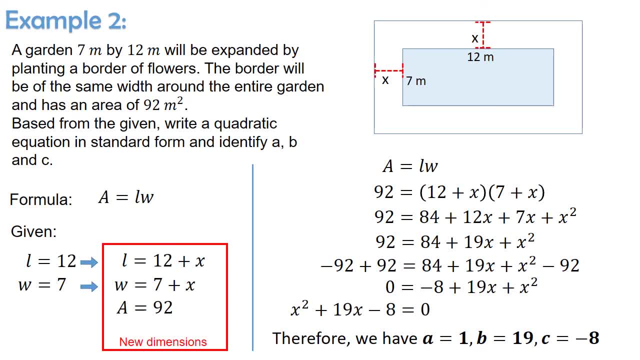 it means its coefficient is 1.. B is equal to 19 and C is equal to negative 8.. Reminders do not disregard the sign before the term. So that's it. We have completed two examples. I hope you learned a lot from our discussion. Thank you for listening.